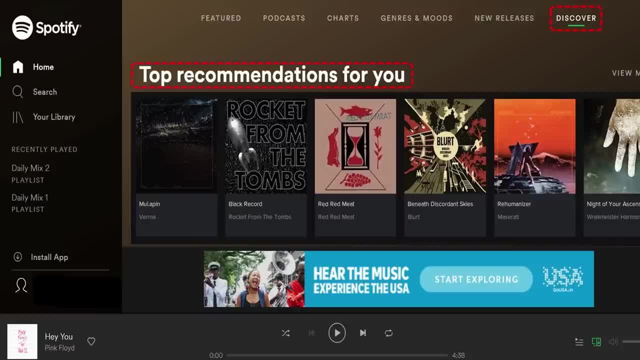 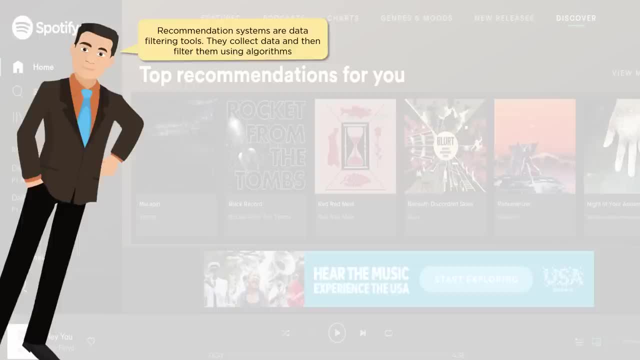 history, like the songs you like listening to and your playlists. This works on something known as the recommendation system. Recommendation systems are nothing but data filtering tools. They collect all the data and then filter them using various algorithms. This system has the ability to accurately predict what a user would like to listen to next, with the 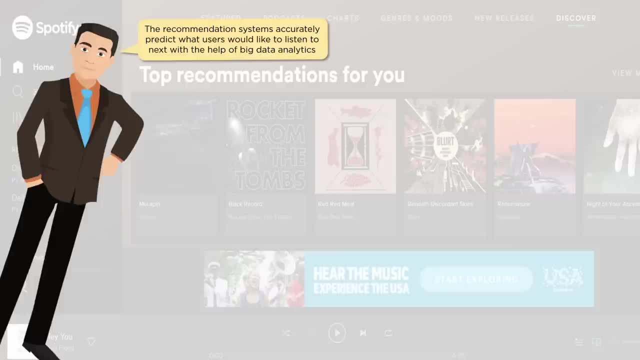 help of Big Data Analytics. This prediction helps the users stay on the page for a longer time, and by doing so, Spotify engages all its users. The users don't have the need to go on searching for different songs. This is because Spotify readily provides them with a variety of songs according to. 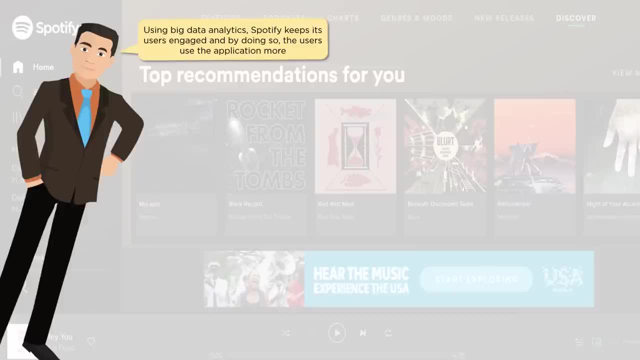 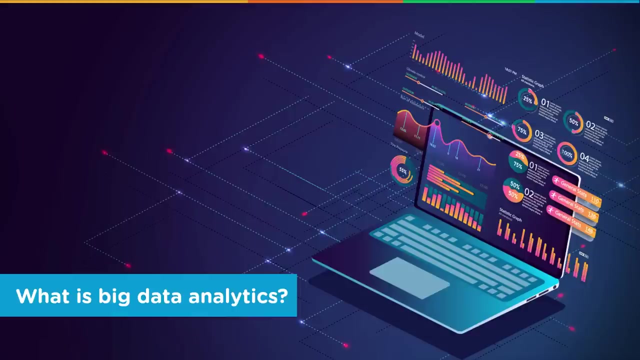 their taste. Well, this is how Big Data Analytics is used by Spotify. Now that we have understood why Big Data Analytics is required, let us move on to our next topic, ie What is Big Data Analytics? But before that, there is another term we need to understand, ie Big Data. We all hear. 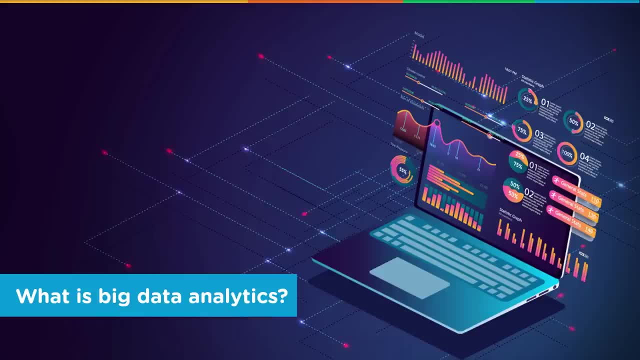 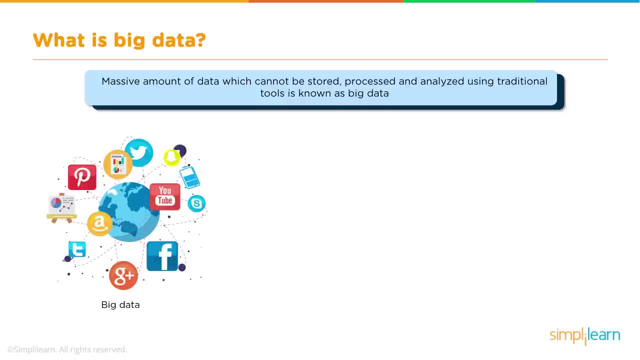 the term Big Data many a times, but do you know what exactly Big Data means? Well, we will understand the term Big Data clearly right now. Big Data is a term for data sets that cannot be handled by traditional computers or tools due to their value, volume, velocity and veracity. It is defined as massive amount of data, which 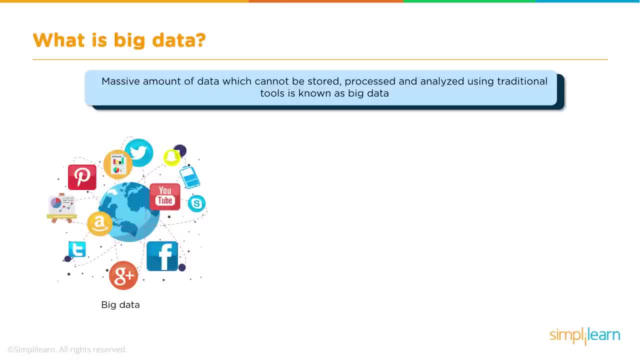 cannot be stored, processed and analysed using various traditional methods. Do you know how much data is being generated every day, every second, Even as I talk right now? there are millions of data sources which generate data at a very rapid rate. These data sources: 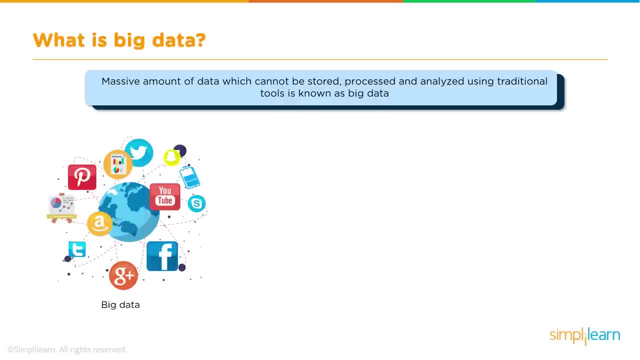 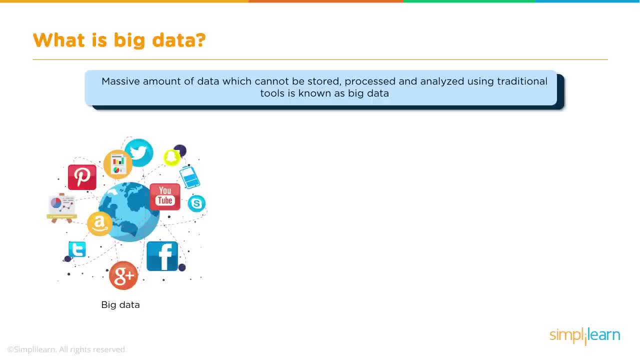 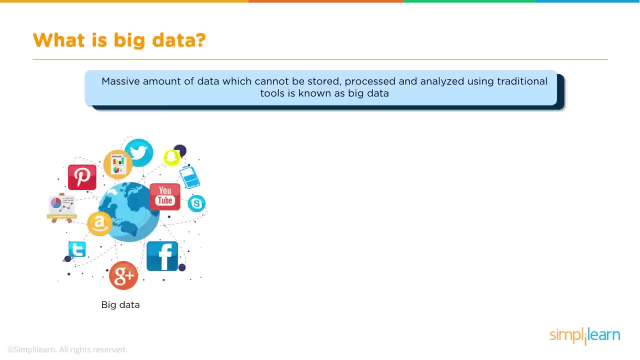 etc. Big Data also contains data of different formats, like structured data, semi structured data and unstructured data. Data like your Excel sheets all fall under structured data. This data has a definite format. Your Email has the fantastical representation of 64 words. 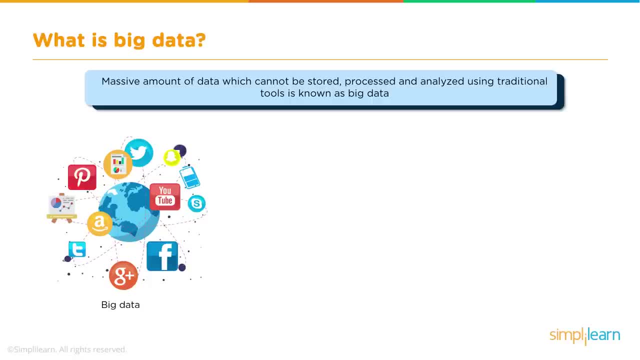 in our text. Banksy has the most image. description of the text, Semistructure of the text, eure images, images and the pictures are all in unstructured format. All these data together make up the formiendoten data, and the information we get from content is completely unstructured. 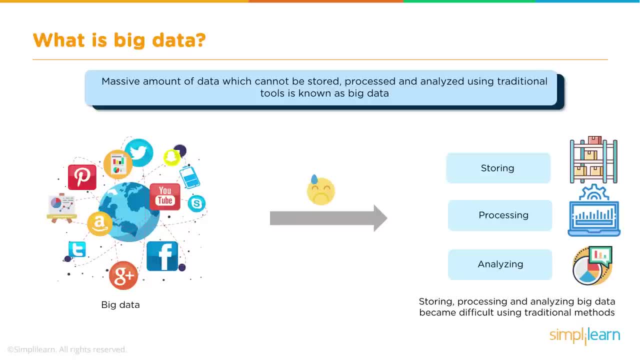 Also, We need ayalog tags, letters and all the other offices和 text. 로 cada thing for big data. It is very tough to store, process and analyze big data using RDBMS. If you have looked into our previous videos, you would know that Hadoop is the solution to this. 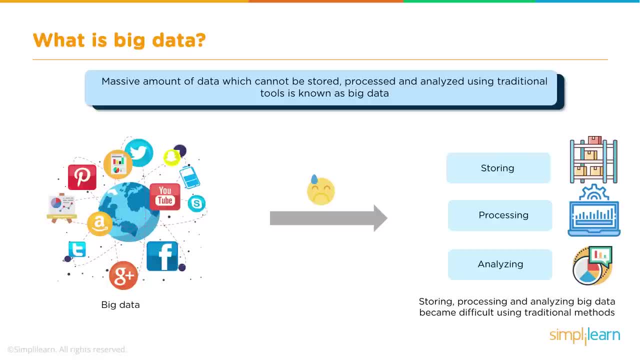 Hadoop is a framework that stores and processes big data. It stores big data using the distributed storage system and it processes big data using the parallel processing method. Hence, storing and processing big data is no more a problem. using Hadoop, Big data in its raw form is: 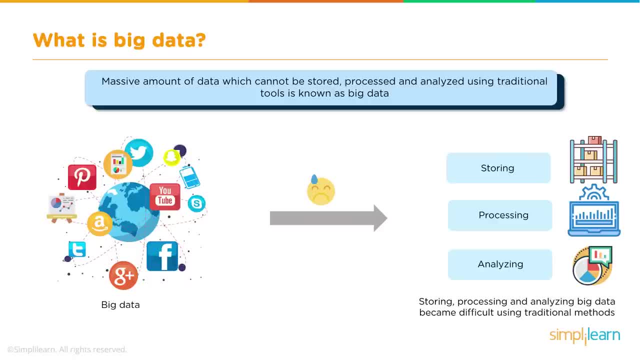 of no use to us. We must try to derive meaningful information from it in order to benefit from this big data. Do you know Amazon uses big data to monitor its items that are in its fulfillment centers across the globe. How do you think Amazon does this? Well, it is. 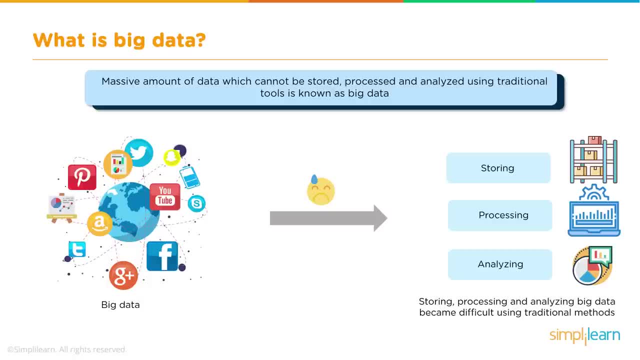 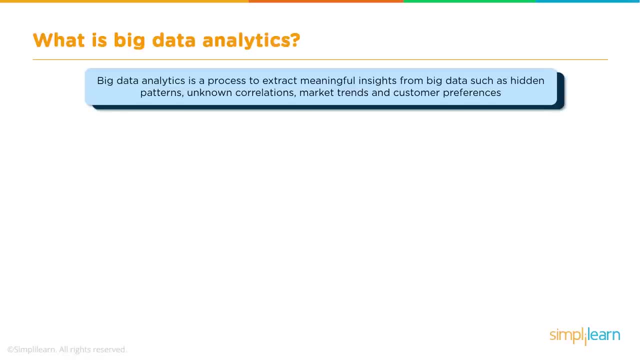 done by analyzing big data, which is known as big data analytics. What is big data analytics? In simple terms, big data analytics is defined as the process which is used to extract meaningful information from big data. This information could be your hidden patterns, unknown correlations. 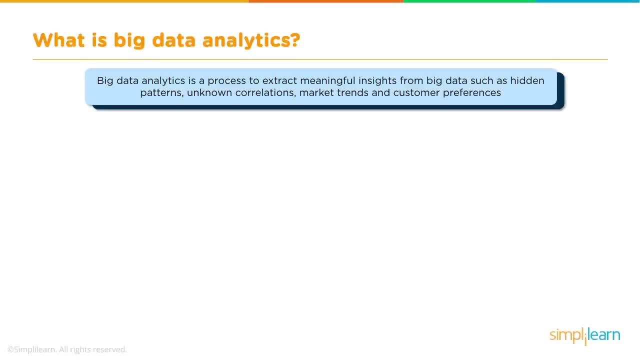 market trends and so on By using big data analytics. there are many advantages: It can be used for better decision making, to prevent fraudulent activities and many others. We will look into four of them step by step. I will first start off with 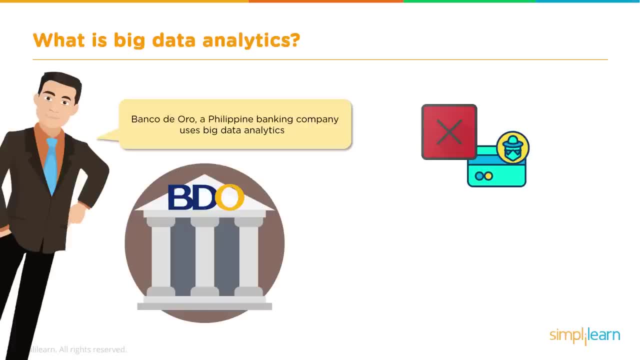 Big Data Analytics which is used for Risk Management. BDO, which is a Philippine banking company, uses Big Data Analytics for risk management. Risk management is an important aspect for any organization, especially in the field of banking. Risk management analysis comprises a series of measures which are employed to: 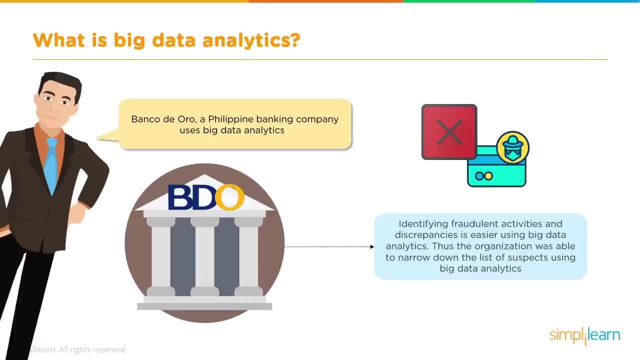 prevent any sort of unauthorized activities. Identifying fraudulent activities was a main concern for BDO. for the bank to identify the fraudster from a long list of suspects, BDO adopted big data analytics which helped the bank to narrow down the entire list of. 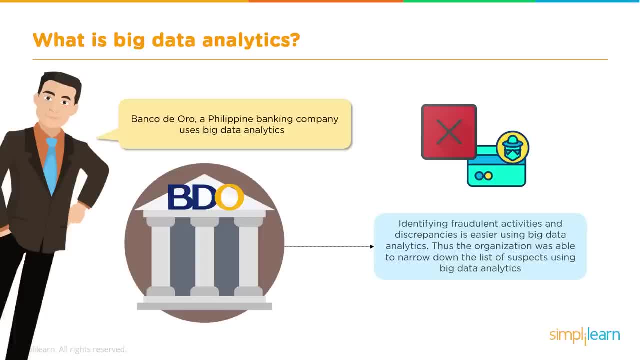 suspects. Thus, the organization was able to identify the fraudster in a very short time. This is how big data analytics is used in the field of banking for risk management. Let us now see how big data analytics is used for product development and innovations with. 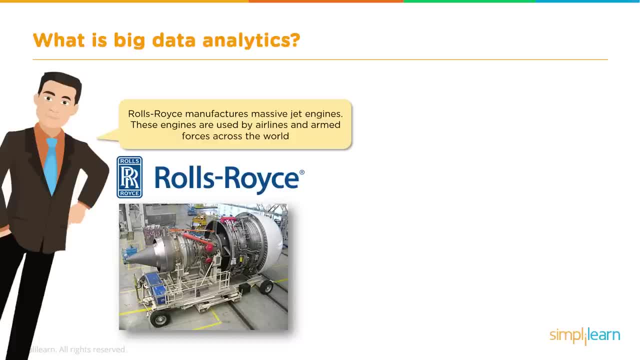 an example. All of you are aware of Rolls Royce cars, right? Do you also know that they manufacture jet engines, which are used across the world? What is more interesting is that they use big data analytics for developing and innovating this engine. 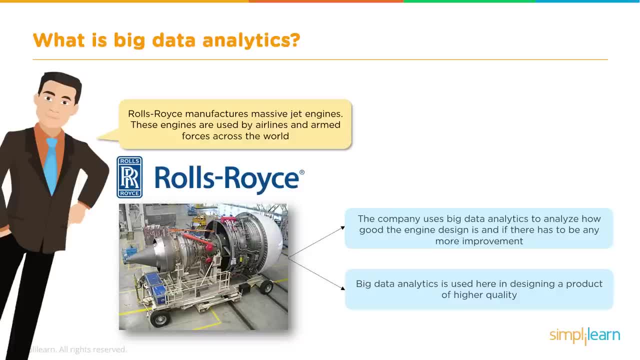 A new product is always developed by trial and error method. Big data analytics is used here to analyze if an engine design is good or bad. It is also used to analyze if there can be more scope for improvement based on the previous models and on the future demands. 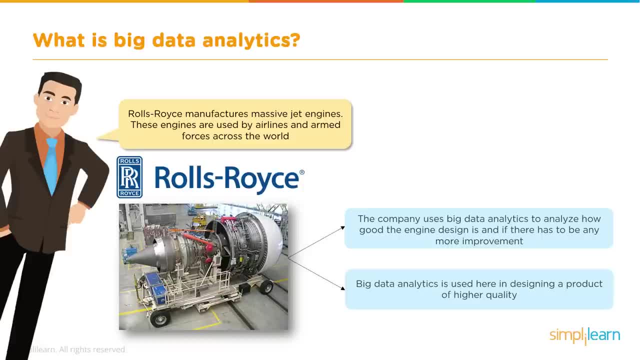 This way, big data analytics is used in designing a product which is of higher quality. Using big data analytics, the company can save a lot of time If the team is struggling to arrive at the right conclusion. big data can be used to zero in on the right data which have to be studied and thus the time spent on the product. 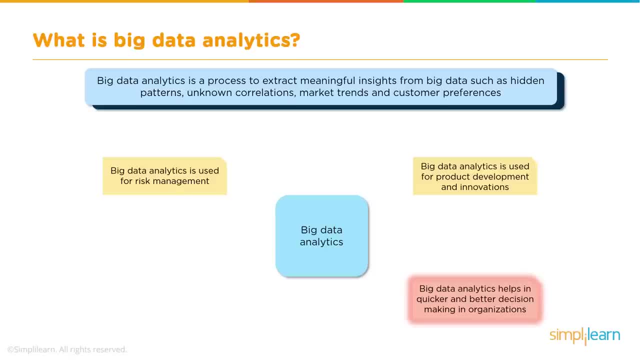 development is less. Big data analytics helps in quicker and better decision making in organizations. The process of selecting a course of analysis is much easier. The process of selecting a course of analysis is much easier. The process of selecting a course of analysis is much easier. 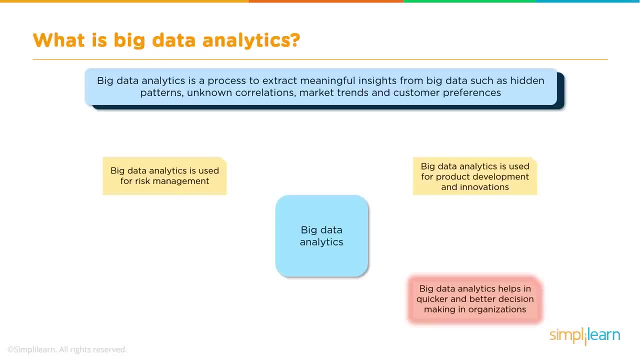 The course of action from various other alternatives is known as decision making. Lot of organizations take important decisions based on the data that they have. Data driven business decisions can make or break a company. Hence it is important to analyze all the possibilities thoroughly and quickly before. 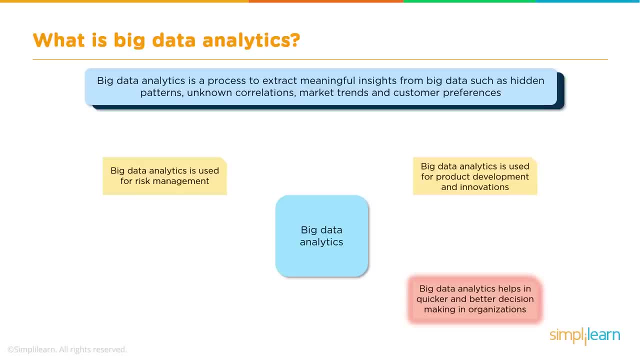 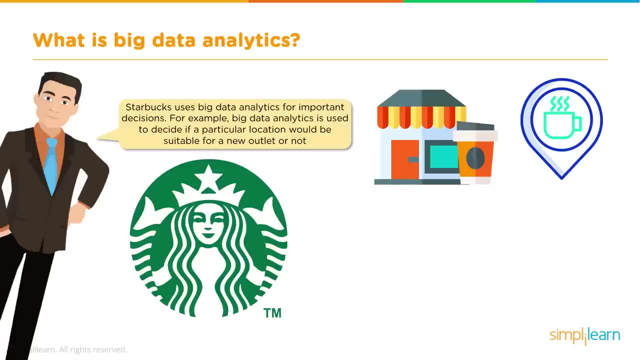 making important decisions. Let us now try to understand this with an use case. Starbucks uses big data analytics for making important decisions. Starbucks uses big data analytics for making important decisions. Starbucks uses big data analytics for making important decisions. The screen is rollable to choose from and the positioning area allows it. 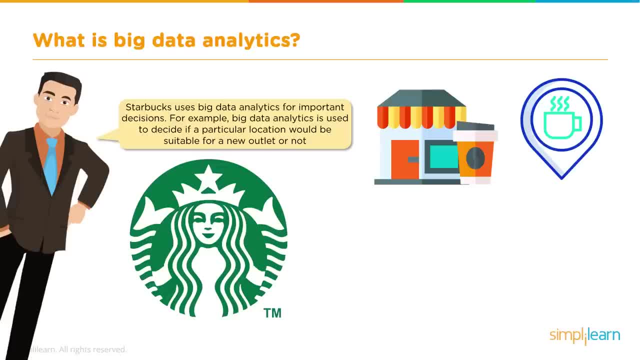 A few miles here or there can always make a huge difference. An verz is the best location to choose at. This also works for other facilities, such as restaurants. Hebrews Project is always open for full uptime and stands here. It clearly indicates that the business is working bumpy. 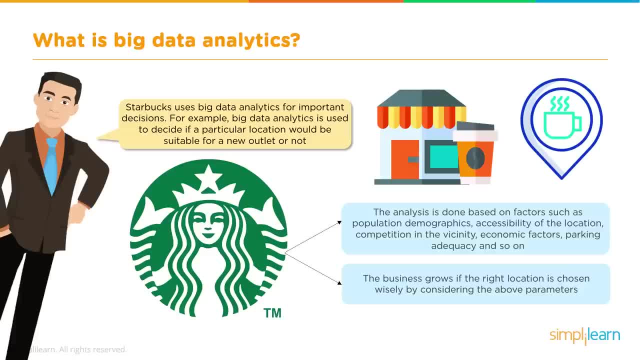 It applies zero to zero consideration. It would be inconvenient for people to go to a store which has no parking facility. Similarly, the other factors that have to be considered are the visibility of the location, the accessibility, the economic factors, the population of that particular location and also 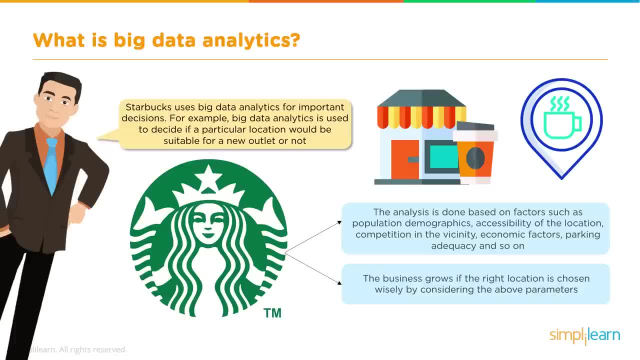 we would have to look into the competition in the vicinity. All these factors have to be thoroughly analysed before making a decision as to where the new outlet must be started. Without analysing these factors, it would be impossible for us to make a wise decision Using big data analytics. 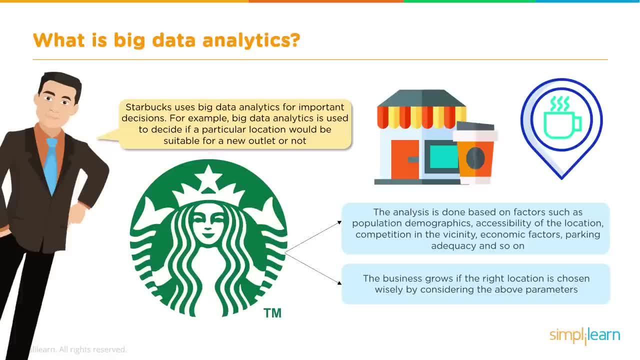 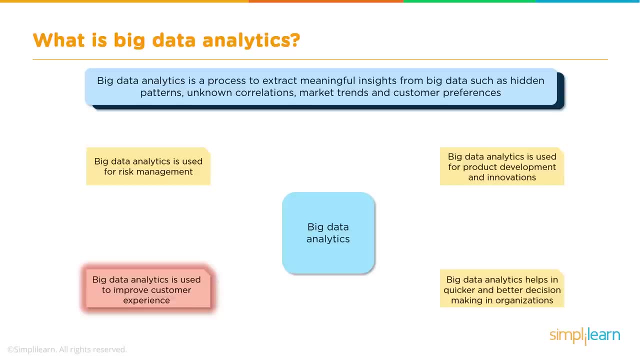 we can consider all these factors and analyse them quickly and thoroughly. Thus, Starbucks makes use of big data analytics to understand if their new location would be fruitful or not. Finally, we will look into how big data analytics is used to improve customer experience using an example. Delta, an American airline, uses big data analytics to improve its customer. 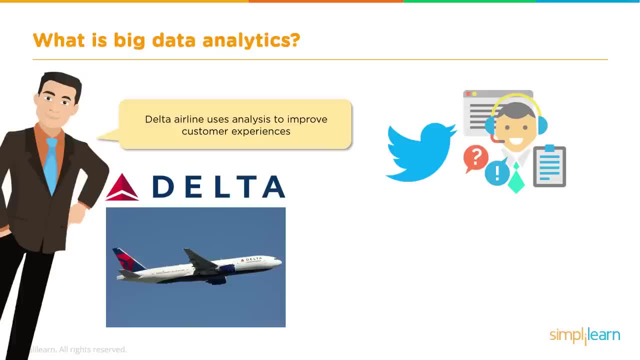 experience. Delta, an American airline, uses big data analytics to improve its customer experience. With the increase in global air travel, it is necessary that an airline does everything they can in order to provide good service and experience to its customers. Delta Airlines improves its. 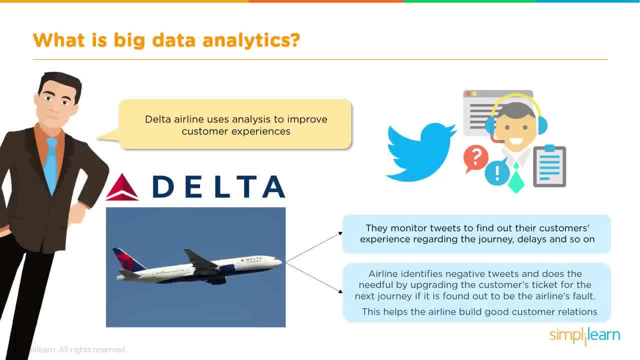 customer experience by making use of big data analytics. This is done by monitoring tweets, which will give them an idea as to how their customer's journey was. If the airline comes across a negative tweet and if it is found to be the airline's fault, the airline goes ahead and 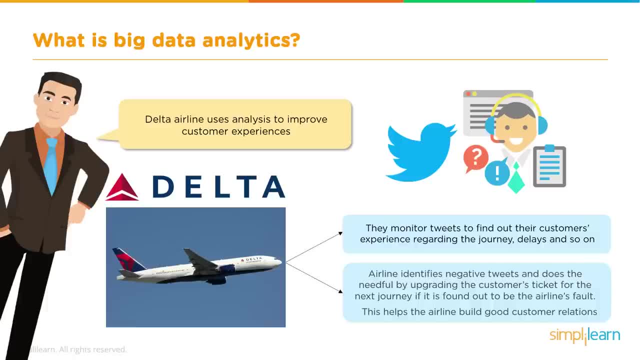 and upgrades that particular customer's ticket. when this happens, the customer is able to trust the airlines and, without a doubt, the customer will choose Delta for their next journey. by doing so, the customer is happy and the airlines will be able to build a good brand recognition. thus we see here that by 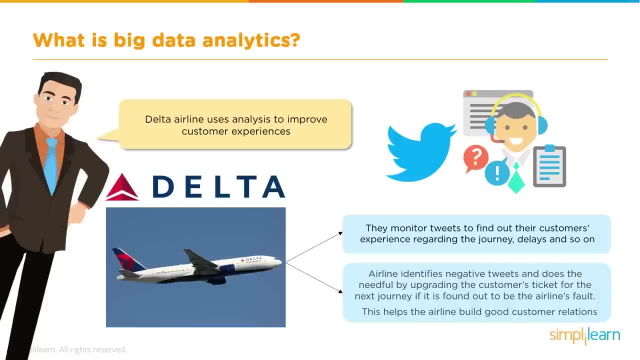 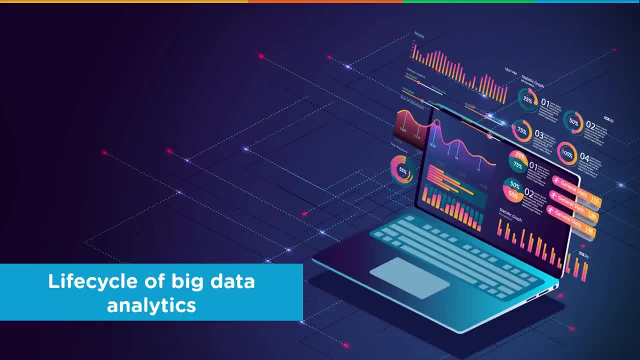 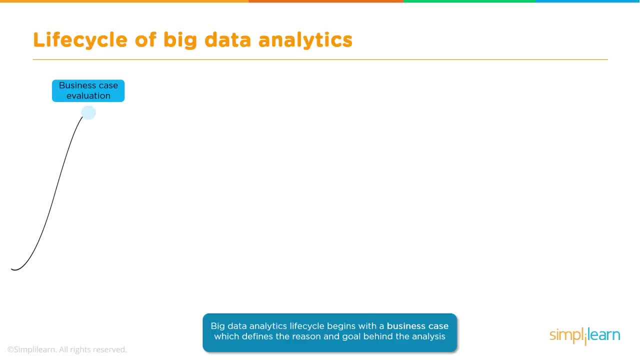 using analysis, Delta Airlines was able to improve its customer experience. moving on to our next topic, that is, lifecycle of big data analytics. here we will look into their various stages as to how data is analyzed from scratch. the first stage is the business case evaluation stage. here, the motor behind 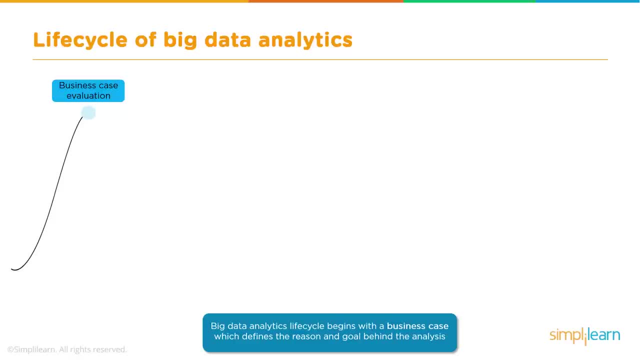 the analysis is identified. we need to understand why we are analysing, so that we know how to do it and what are the different parameters that have to be looked into. once this is done, it is clear for us and it becomes clear to us. Thank you, bajita. why are these analytics and how are they applied? 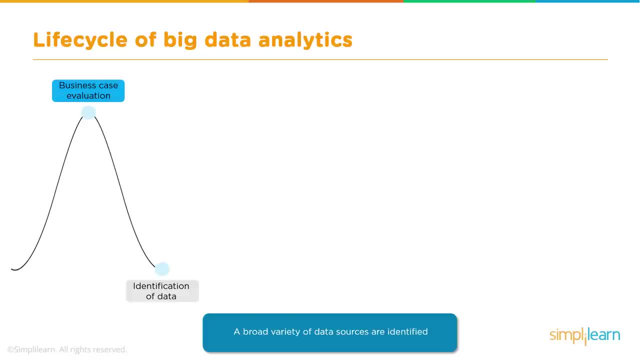 much easier for us to proceed with the rest, after which we will look into the various data sources from where we can gather all the data which will be required for analysis. once we get the required data, we will have to see if the data that we received is fit for analysis or not. not all the data that we 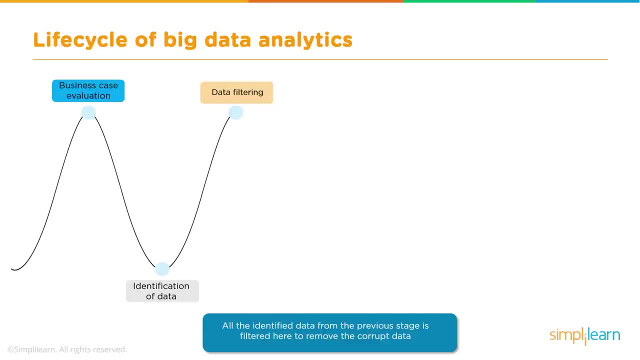 receive will have meaningful information. some of it will surely just be corrupt data. to remove this corrupt data, we will pass this entire data through a filtering stage. in this stage, all the corrupt data will be removed. now we have the data minus the corrupt data. do you think our data is now fit for analysis? 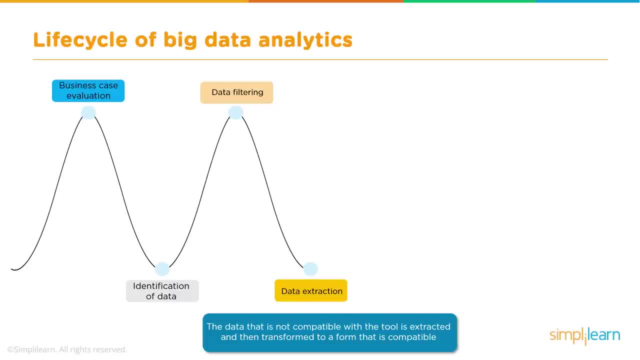 well, it is not. we still have to figure out which data will be compatible with the tool that we will be using for analysis. if we find data which is incompatible, we first extract it and then transform it to a compatible form, depending on the tool that we use. in the next stage, all the data with the 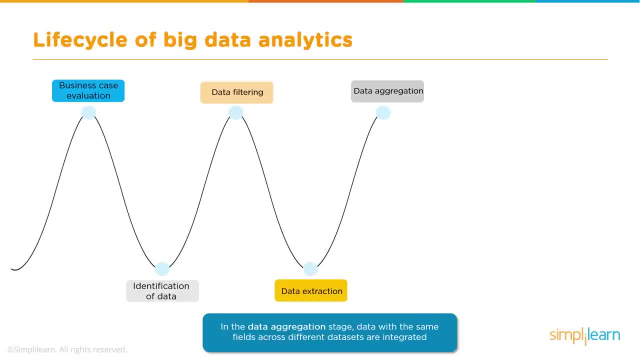 same fields will be integrated. this is known as the data aggregation stage. the next stage, which is the analysis stage, is a very important stage in the lifecycle of big data analytics. right here in this step, the entire process of evaluating your data using various analytical and statistical tools to 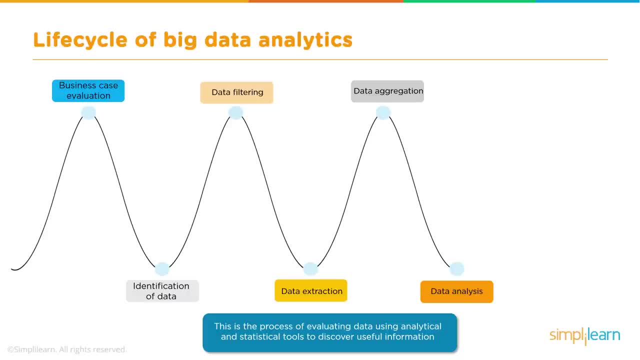 discover meaningful information is done. like we have discussed before, the entire process of deriving meaningful information from data, which is known as analysis, is done here in this stage. the result of the data analysis stage is then graphically communicated using tools like tableau power bi clickview. this analysis result will then be made. 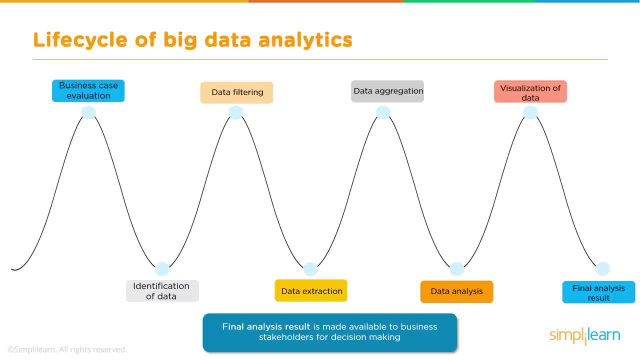 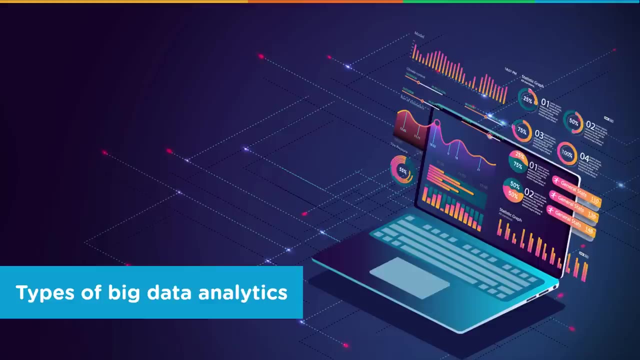 available to different business stakeholders for various decision-making. this was the entire lifecycle of big data analytics. we just saw how data is analyzed from scratch. now we will move on to a very important topic, that is, the different types of big data analytics. well, we have four different types of big data analytics, as you see here. these are: 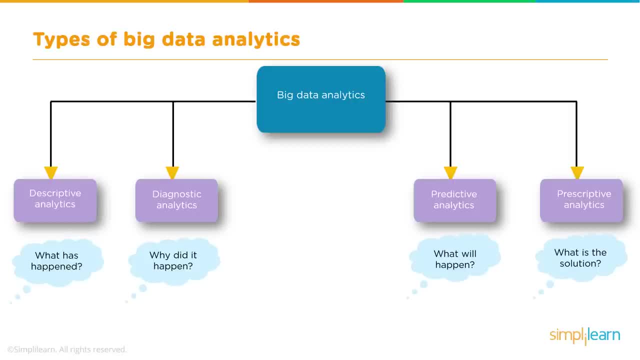 the types, and below this are the questions that each type tries to answer. we have descriptive analytics, which asks the question: what has happened? then we have diagnostic analytics, which asks: why did it happen. predictive analytics, asking what will happen. and prescriptive analytics, which questions by asking what is the solution. we will look into all these four, one by 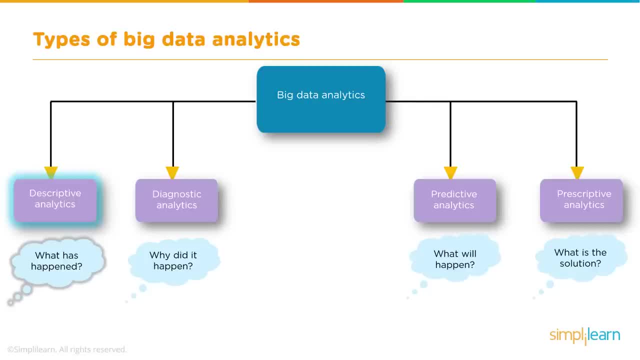 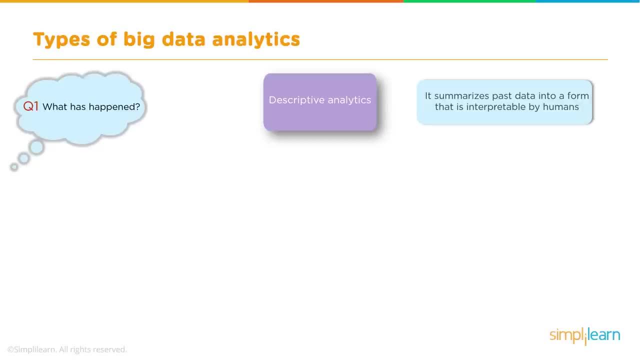 one with an use case for each. we will first start off with descriptive analytics. as mentioned earlier, descriptive analytics asks the question: what has happened? it can be defined as the type that summarizes past data into a form that can be understood by humans. in this type, we will look at the type of 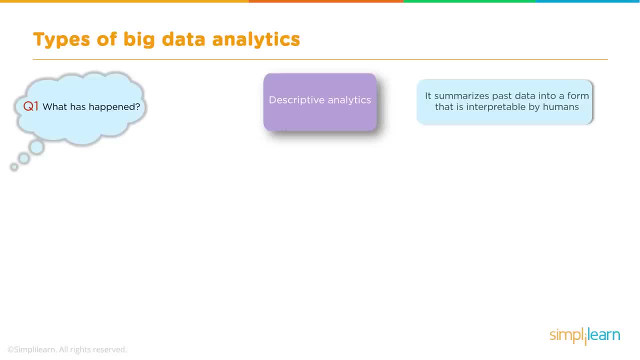 data. we will look into the past data and arrive at various conclusions. for example, an organization can review its performance using descriptive analytics, that is, it analyzes its past data, such as revenue over the years, and arrives at a conclusion with the profit. by looking at this graph, we can understand if the 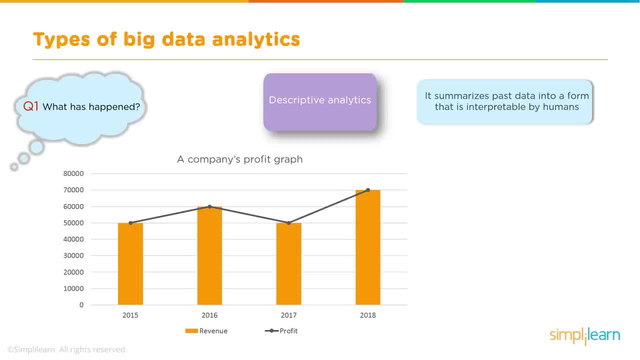 company is running at a profit or not. thus, descriptive analytics helps us understand this easily. we can simply say that descriptive analytics is used for creating various reports for companies and also for tabulating various social media metrics like Facebook likes, tweets, etc. now that we have seen what is descriptive analytics, let us look into and use case. 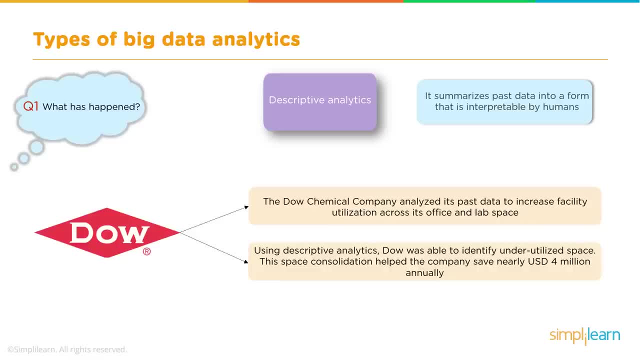 of descriptive analytics. the Dow Chemical Company analyzed all its past data using descriptive analytics and by doing so they were able to identify the underutilized space in their facility. descriptive analytics helped them in this space consolidation. on the whole, the company was able to save nearly 4 million dollars annually. so we now see here that descriptive analytics 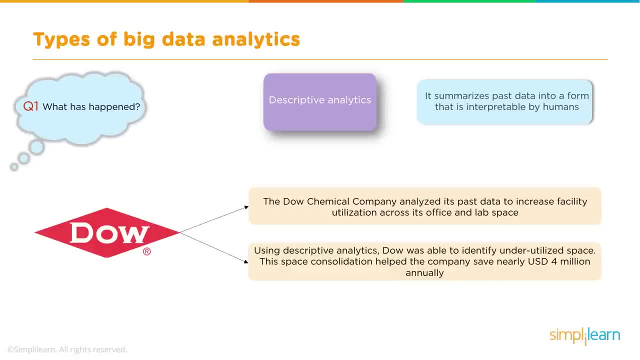 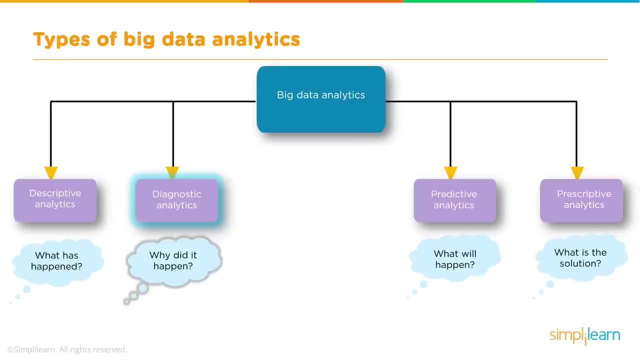 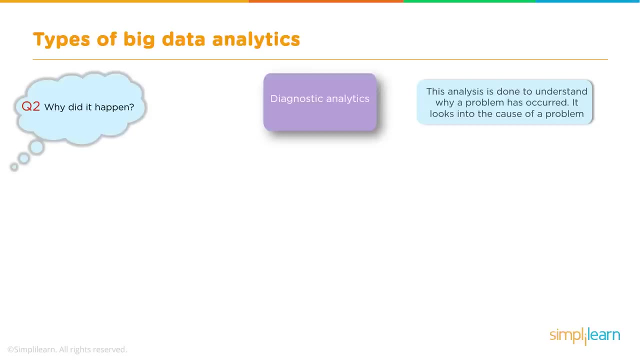 not only helps us derive meaningful information from the past data, but it can also help companies in cost reduction if it is used wisely. let us now move on to our next type, that is, diagnostic analytics. diagnostic analytics asks the question why a particular problem has occurred. as you can see, it will always ask the question: why did it happen? it will look. 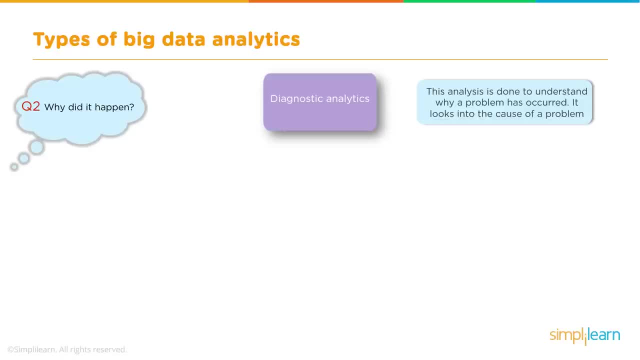 into the root cause of a problem and try to understand why it has occurred. diagnostic analytics makes use of various techniques such as data mining, data discovery and drilldown. companies benefit from this type of analytics because it helps them look into the root cause of a problem. by doing so, the next 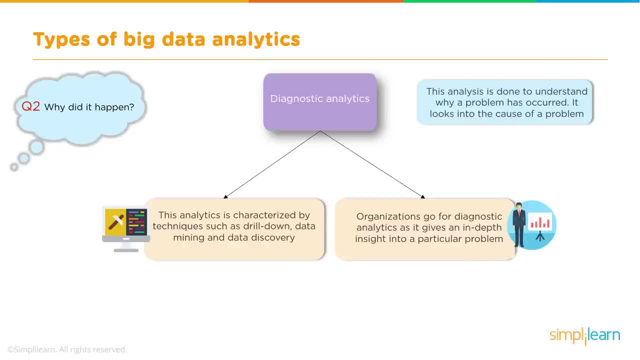 time the same problem will not arise, as the company already knows why it has happened and they will at a particular solution for it. Inetsoft's BI Query Tool is an example of Diagnostic Analytics. We can use Query Tool for Diagnostic Analytics, Now that you know why Diagnostic Analytics is required and what Diagnostic Analytics 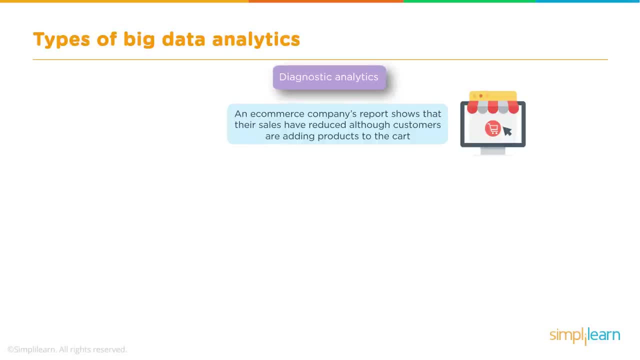 is. I will run you through an example which shows where Diagnostic Analytics can be used. All of us shop on e-commerce sites, right? Have you ever added items to your cart but ended up not buying it? Yes, all of us might have done that at some point. 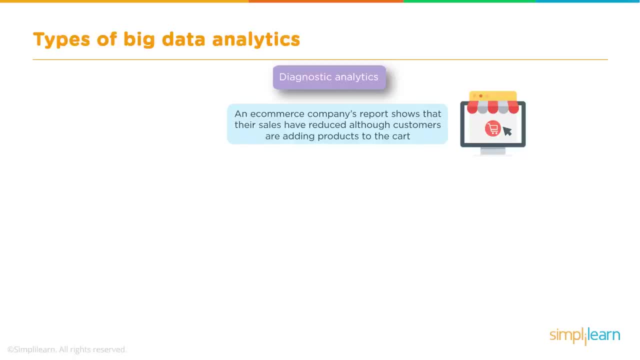 An organization tries to understand why its customers don't end up buying their products, although it has been added to their carts, And this understanding is done with the help of Diagnostic Analytics. An e-commerce site wonders why they have made few online sales, although they have had a. 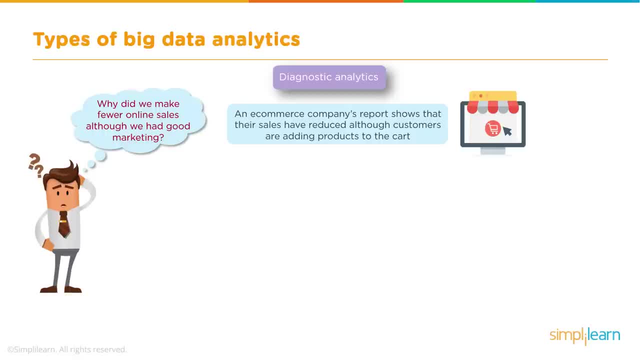 very good marketing strategy. There could have been various factors as to why this has happened, Factors like the shipping fee, which was too high, Or the page that was sold out That didn't load correctly, Not enough payment options available, and so on. 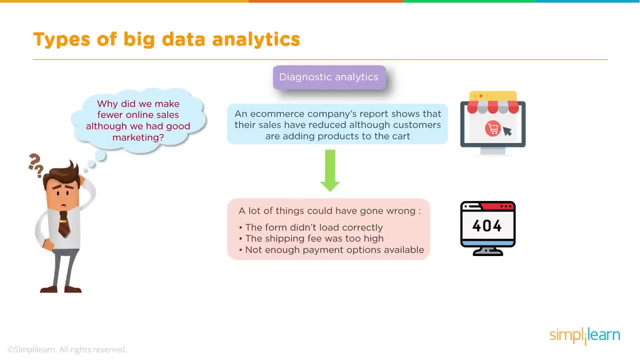 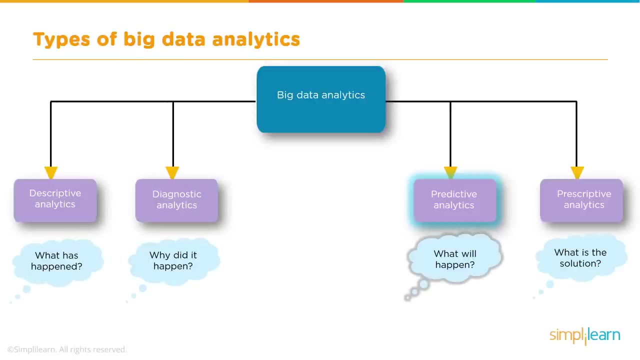 All these factors are analyzed using Diagnostic Analytics and the company comes to a conclusion as to why this has happened. Thus we see here that the root cause is identified, so that in future the same problem doesn't occur again. Let us now move on to the third type, that is, Predictive Analytics. 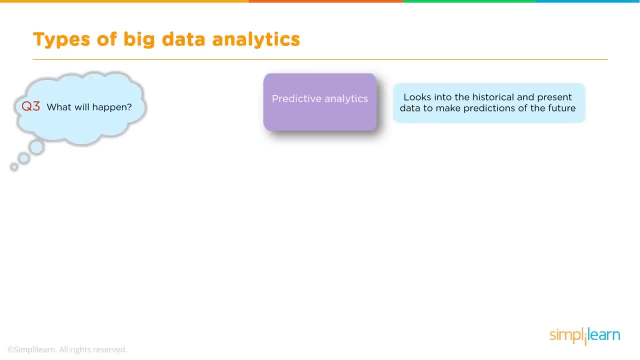 As the name suggests, Predictive Analytics makes predictions of the future. It analyzes the current and historical data. It analyzes the current and historical data. It uses historical facts to make predictions about future. It always asks the question: what will happen next? Predictive Analytics is used with the help of artificial intelligence, machine learning. 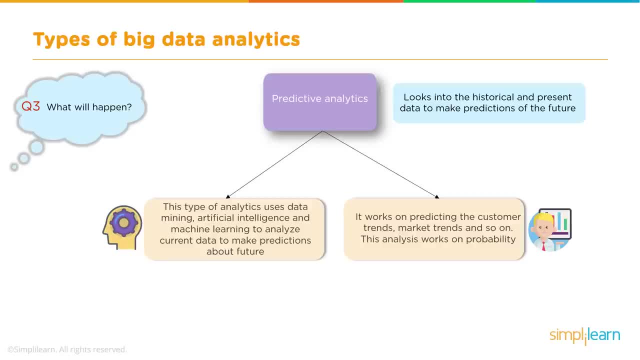 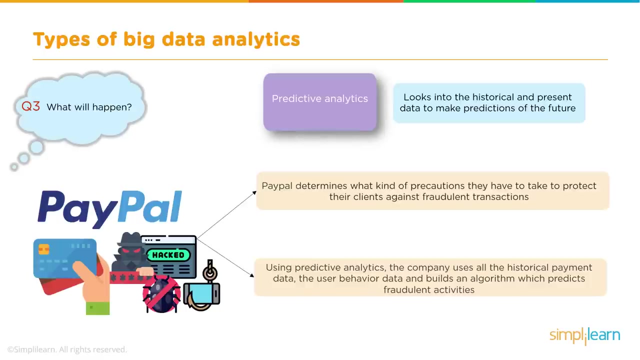 data mining to analyze the data. It can be used for predicting customer trends, market trends, customer behavior, etc. It solely works on probability. It always tries to understand what can happen next with the help of all the past and current information. It is very frustrating that only one possibility is met and one or more of those possibilities. 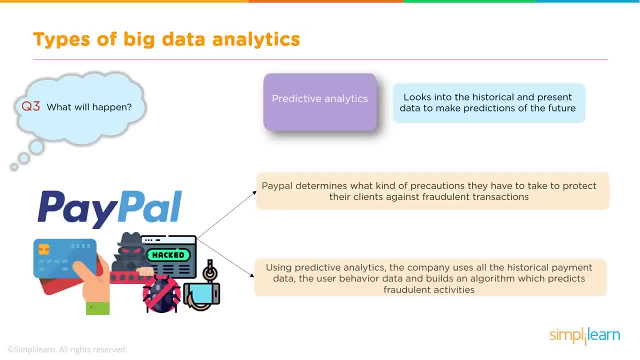 cannot be estimated. Whendecidive Analytics can provide self-indiedo, It makes the테 ин忘, even if its data is established within a Council. However, when it comes to Predictive Analytics, it is andar. It doesn't justify policy revens and various other things, but Some criteria are always. 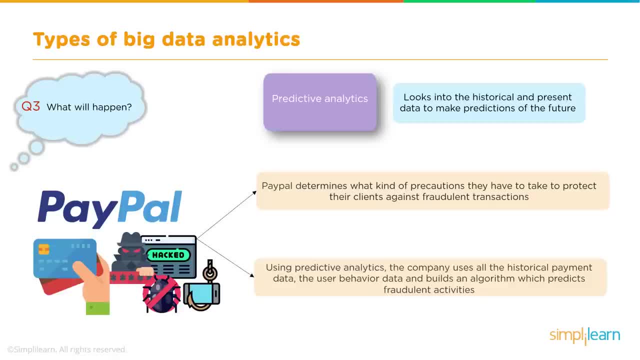 used, For example, drugs, drugs, PayPal, which is one of the largest online payment processors in the world. But PayPal uses analytics wisely here to prevent such fraudulent activities and to minimize them. It uses predictive analytics to do so. The organization is able to analyze past data, which includes a customer's historical payment. 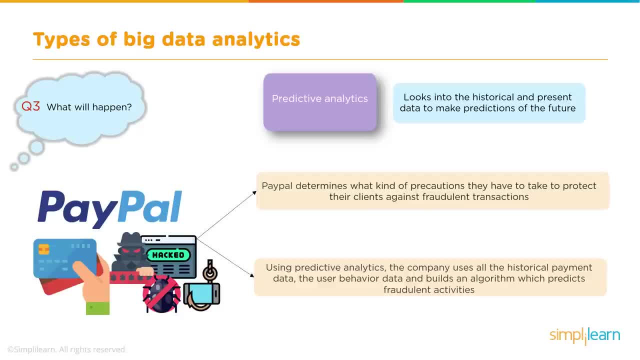 data, a customer's behavior trend, and then it builds an algorithm which works on predicting what is likely to happen next with respect to their transaction. With the use of big data and algorithms, the system can gauge which of the transactions are valid and which could be potentially a fraudulent activity. 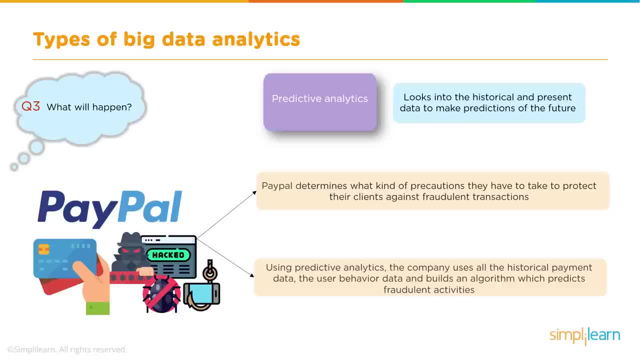 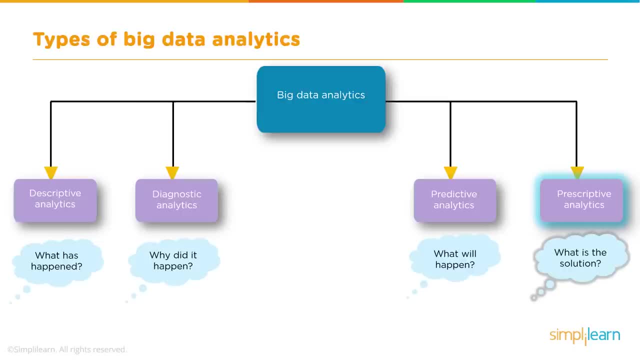 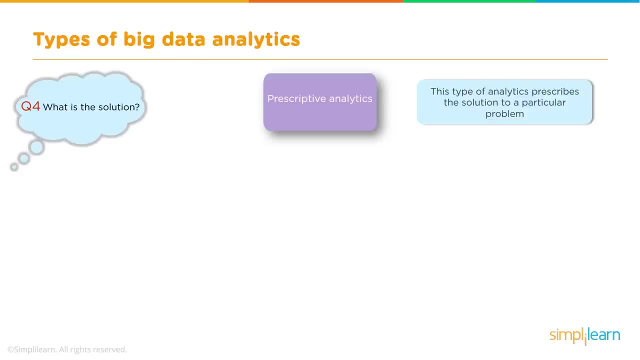 By doing so, PayPal is always ready with precautions that they have to take to protect all their clients against fraudulent transactions. We will now move on to our last type, that is, Prescriptive Analytics. Prescriptive Analytics, as the name suggests, always prescribes a solution to a particular problem. 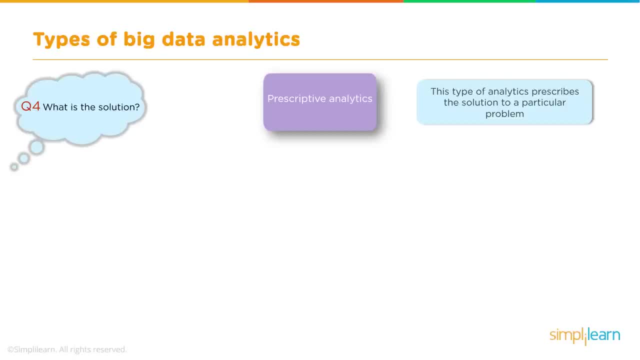 The problem can be something which is happening currently. Hence it can be termed as the type that always asks the question: what is the solution? Prescriptive Analytics is related to both Predictive and Descriptive Analytics, As we saw earlier. Descriptive Analytics always asks the question: what has happened? 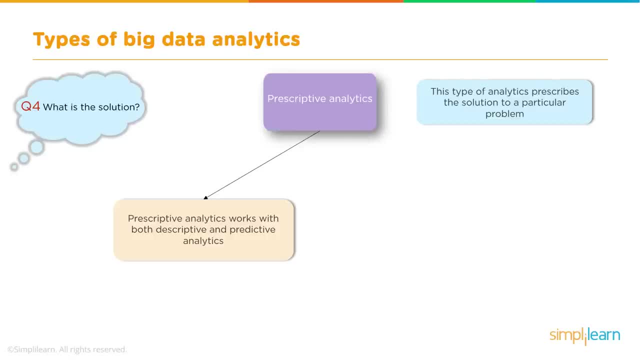 And Predictive Analytics helps you understand what can happen next. With the help of artificial intelligence and machine learning, Prescriptive Analytics helps you arrive at the best solution for a particular problem. Various business rules, algorithms and computational modeling procedures are used in Prescriptive. 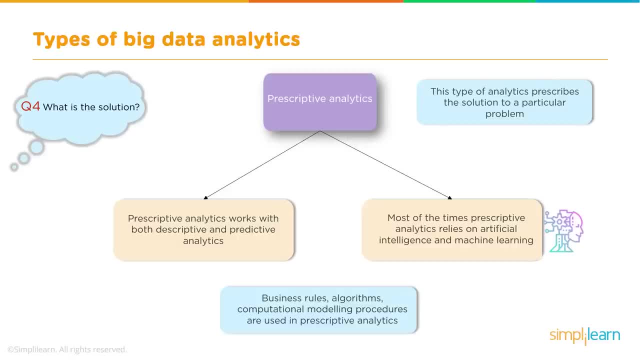 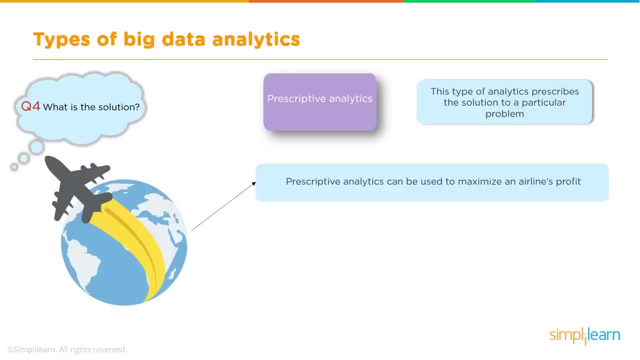 Analytics. Let us now have a look at how and where Prescriptive Analytics is used. with an example Here we will understand how Prescriptive Analytics is used by an airline for its profit. Do you know that when you book a flight ticket, the price of it depends on various factors? 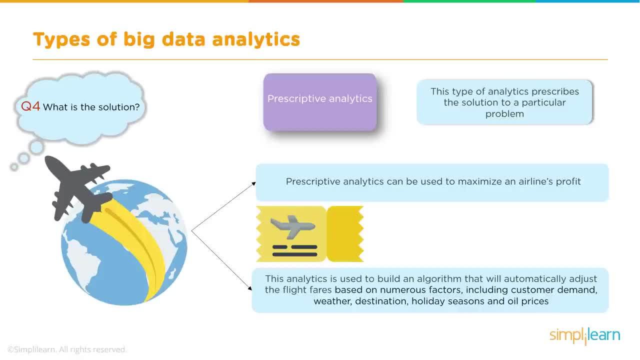 both internal and external? Do you know that when you book a flight ticket, the price of it depends on various factors, both internal and external, and external factors? Apart from taxes, seat selection, there are other factors like oil prices, customer demand, which are all taken into consideration before the flights fare is displayed. Prices change due to availability and demand. Holiday seasons are a time when the rates are much higher than the normal days- Seasons like Christmas and school vacations. also weekends, the rates will be much higher than weekdays. Another factor which determines a flights fare is your destination. Depending on the place where you are travelling to, the flight fare. 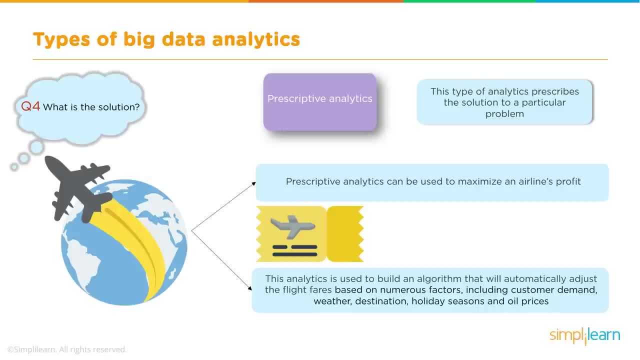 will be adjusted accordingly. This is because there are quite a few places where the air traffic is less, and in such places the flights fare will also be less. So prescriptive analytics analyses all these factors that are discussed and it builds an algorithm which will automatically. 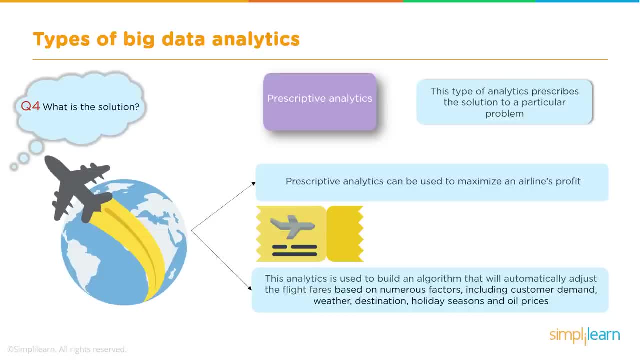 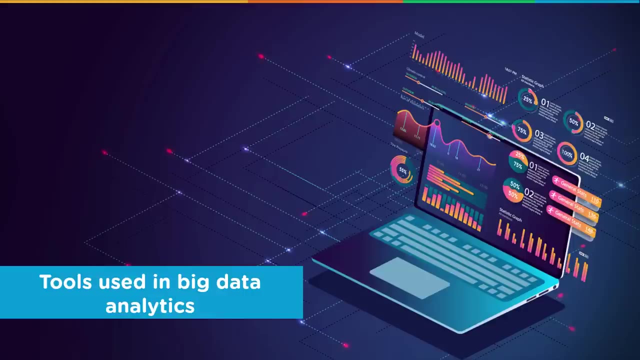 adjust a flights fare. By doing so, the airline is able to maximize its profit. These were the four factors that are discussed in this video. Now let us understand how we achieve these with the use of big data tools. Our next topic will be the various tools used in big data analytics. These are a few of the tools that 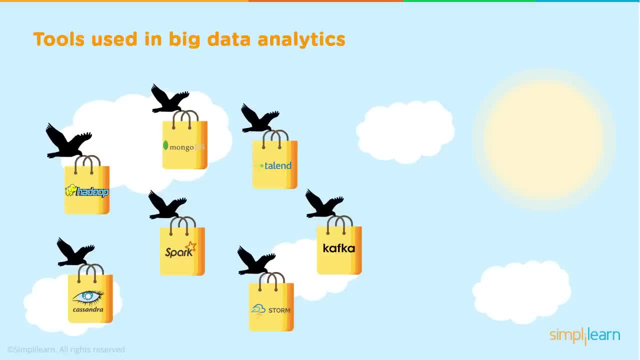 I will be talking about today. We have Hadoop, MongoDB, Talendee, Kafka, Cassandra, Spark and Storm. We will look into each one of them one by one. We will first start off with Hadoop. When you speak of big data, the first framework that comes into everyone's mind is: 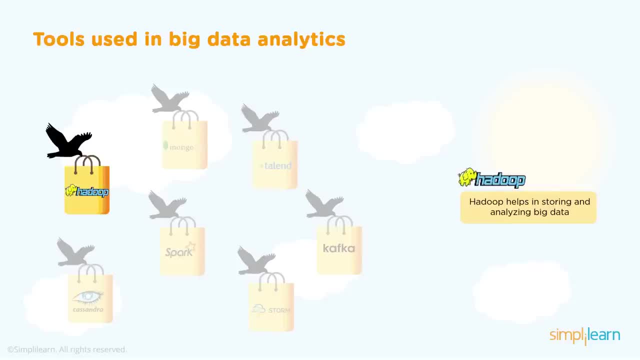 Hadoop, isn't it? As I mentioned earlier, Apache Hadoop is used to store and process big data in a distributed and parallel fashion. It allows us to process data very fast. Hadoop uses MapReduce, Pig and Hive for analyzing this big data. Hadoop is easily one of the 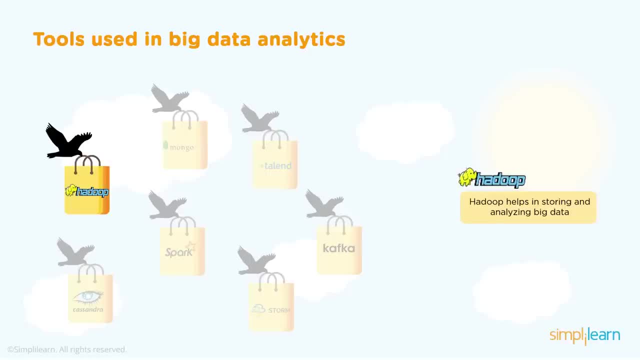 most famous big data tools. Now let us move on to the next one, that is MongoDB. MongoDB is a cross-platform document-oriented database. It has the ability to store and process big data. It has the ability to deal with large amount of unstructured data. Processing of 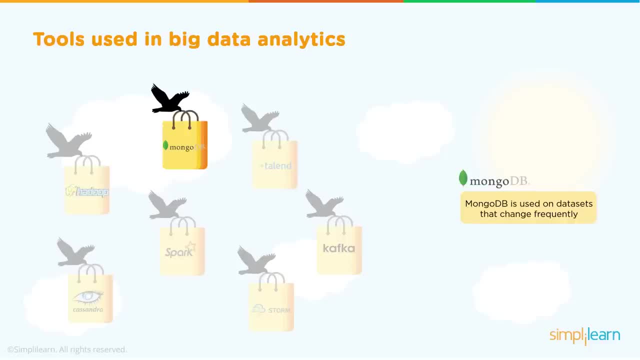 data, which is unstructured, and processing of data sets that change very frequently is done using MongoDB. Talendee provides software and services for data integration, data management and cloud storage. It specializes in big data integration. Talendee Open Studio is a free 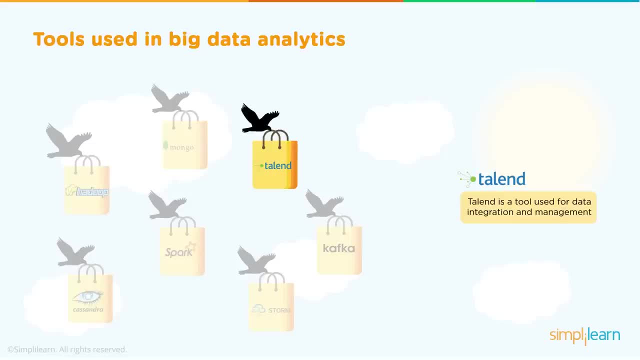 open source tool for processing data easily on a big data environment. Cassandra is the main one. Cassandra is used widely for an effective management of large amounts of data. It is similar to Hadoop in its feature of fault tolerance, where data is automatically replicated to multiple nodes. Cassandra is preferred for real-time processing- Spark. 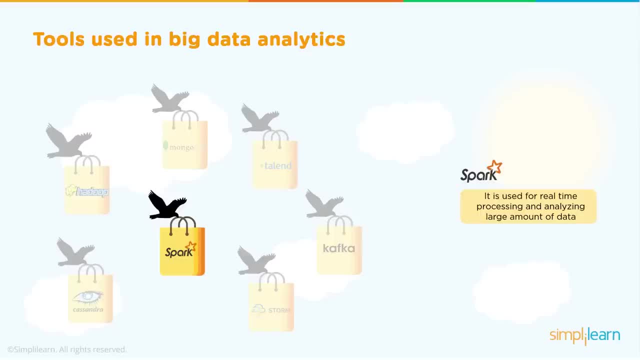 is another tool that is used for data processing. This data processing engine is developed to process data way faster than Hadoop MapReduce. This is done in a way because Spark does all the processing in the main memory of Hadoop Storm is a free big data computational system which is done in real-time. It is one of the 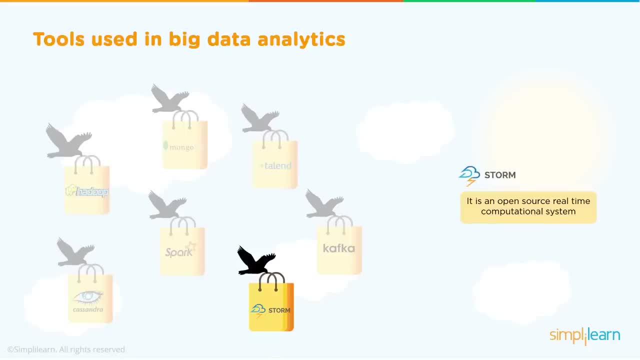 easiest tools for big data analysis. It can be used with any programming language. This feature makes Storm very simple to use. Finally, we will look into another big data tool which is known as Kafka. Kafka is a distributed streaming platform which was developed by LinkedIn and later given to Apache Software. 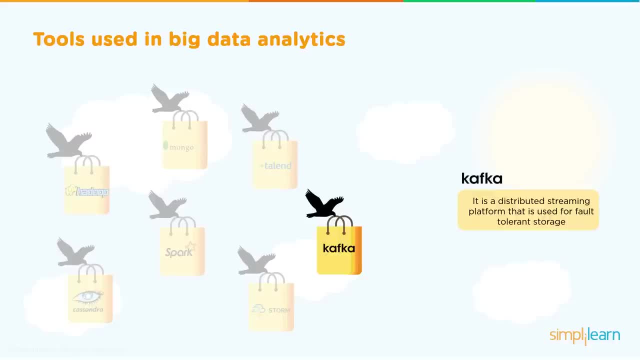 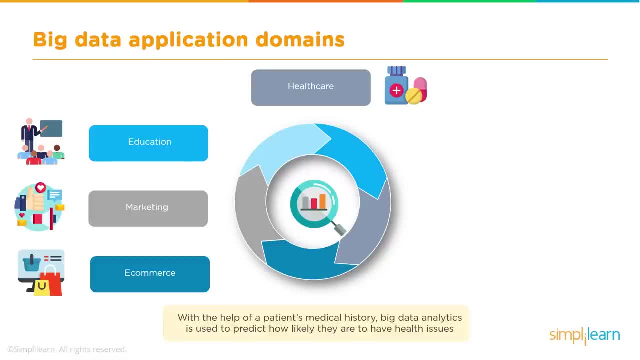 the various sectors where big data application domains can be used. Here we will look into likely they are to have a particular health issue in the future. the example of Spotify that we saw previously showed how big data analytics is used to provide a personalized recommendation list to all its users. similarly, in the 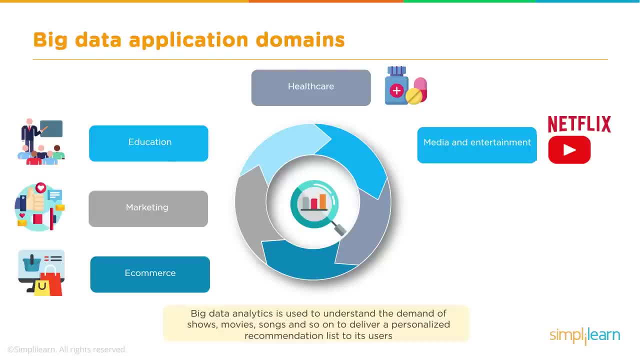 field of media and entertainment. big data analytics is used to understand the demands of shows, songs, movies and so on, to deliver personalized recommendation lists, as we saw with Spotify. big data analytics is used in the field of banking, as we saw previously. with a few use cases, big data analytics was used. 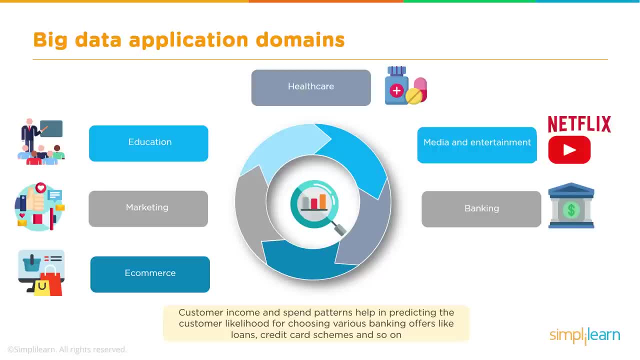 for risk management. in addition to risk management, it is also used to analyze a customer's income and spend patterns and to help the bank predict if a particular customer is going to choose any of the bank offers, such as loans, credit cards schemes and so on. this way, the bank is able to identify the right customer who. 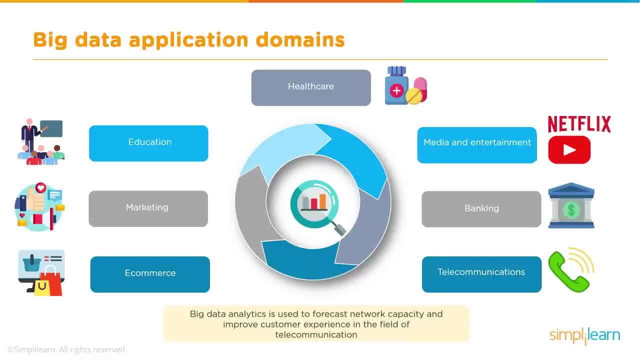 is interested in its offers. it has noticed that technology is becoming more popular, and so is the market economy, and so communities are. Com companies have begun to embrace big data to gain profit. big data analytics helps in analyzing network traffic and call data records. it can also improve.